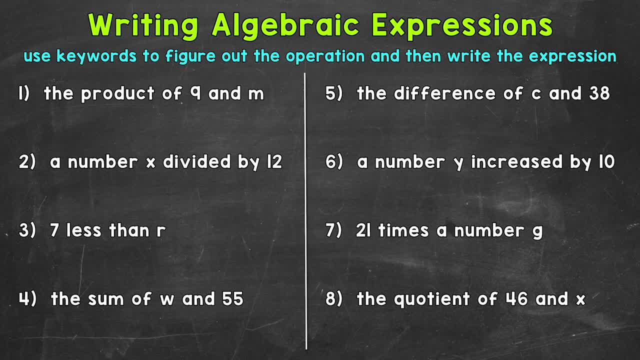 and really a solid foundation for all of math, Because taking these phrases and being able to understand them helps us to apply math and the correct operation to situations. So this is a key skill in algebra and problem solving And, most importantly, problem solving situations in real life where math is applied. 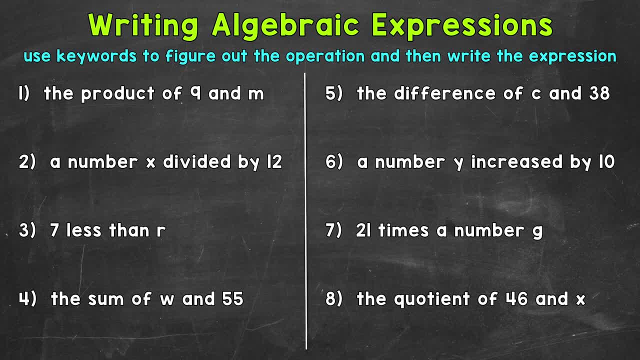 Now, recognizing keywords is going going to be extremely important when writing algebraic expressions. So let's jump into our examples and start with number one, where we have the product of 9 and m. So product is going to be our keyword. 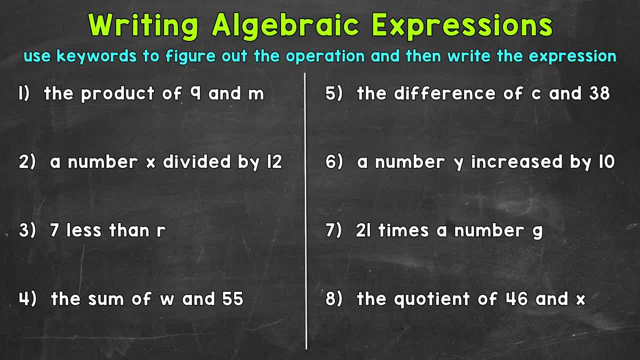 It means the answer to a multiplication problem. So we know this is going to be multiplication 9 times m. Now m is our variable. It's a letter that represents a value we do not know yet, so an unknown. Let's go through some different ways that we can write algebraic expressions that involve multiplication. 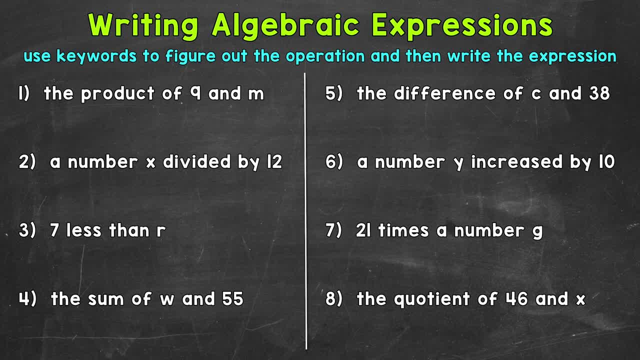 Now this first one we want to avoid, and that's using an x to represent our multiplication symbol. Now, we want to avoid this so we don't have any confusion, because this can mean two things: 9xm, where we have an algebraic expression with two variables, x and m. 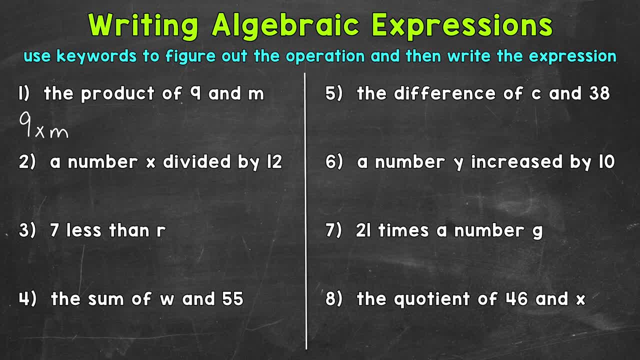 Or does it mean 9 times m? So let's avoid using that. Our other options? well, the first one we can use 9m. So a number next to a variable represents multiplication. Another option would be using an x to represent multiplication. 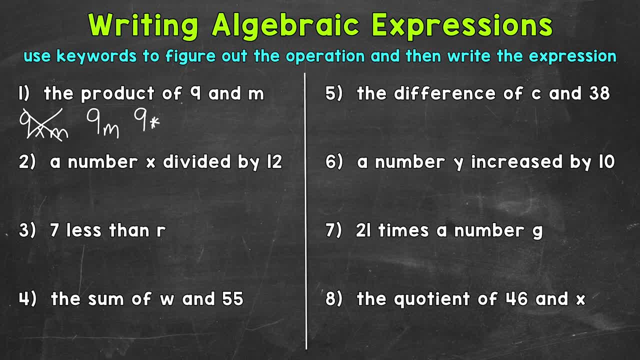 An asterisk, so something that looks like this represents multiplication as well. Another option, using a filled in circle or dot, represents multiplication. And then, lastly, we can use parentheses, So anytime we have a number next to parentheses, that represents multiplication as well. 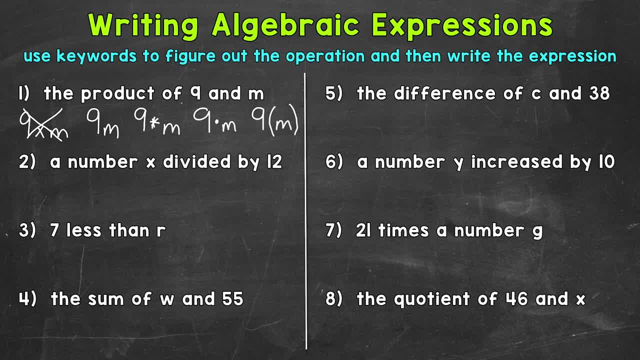 Let's move on to number 2, where we have a number, x divided by 12.. So this is going to be division. So we can write this out: x divided by 12.. We can do x divided by 12.. Or we can do a slash: x divided by 12.. 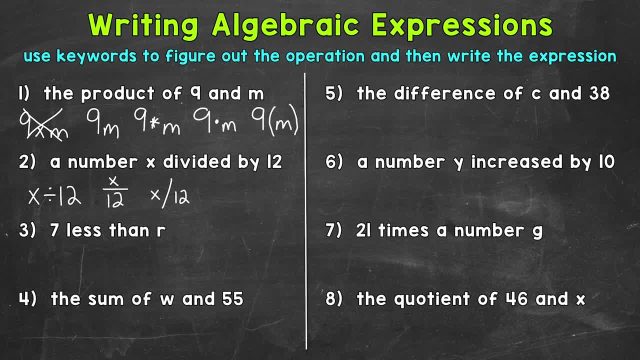 So some different options for division as well. Number 3,: 7 less than r. Now this one: we switched the order And we need to think less than We are taking: 7 less than r. So this is going to be subtraction. 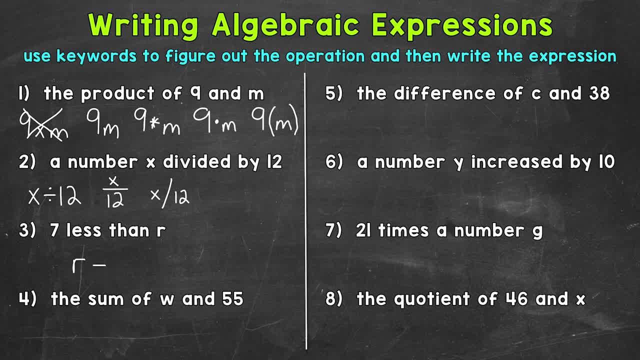 And it's going to be r minus 7 less than So. whenever we see less than, we actually switch the order. So the r comes first and the 7 comes second. We are taking 7 less than that r, So switch that order. 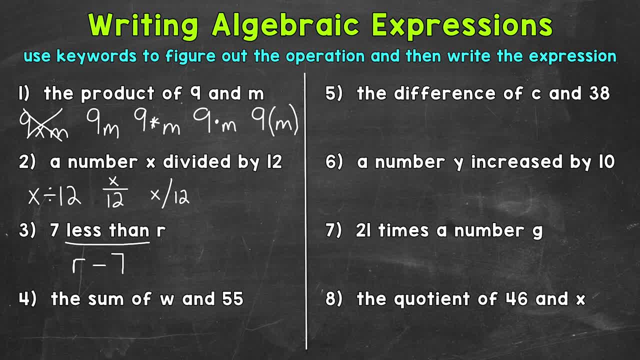 Number 4, the sum of w and 55. So sum is our key word there And that's the answer to an addition problem. So this is going to be addition w plus 55.. On to number 5, where we have the difference of c and 38. 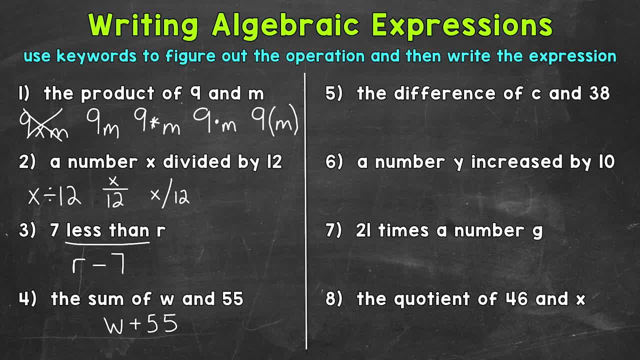 So our key word difference? well, that's the answer to a subtraction problem. So this is going to be subtraction c minus 38.. So in the case of that subtraction algebraic expression, we keep the order c first, 38 second. 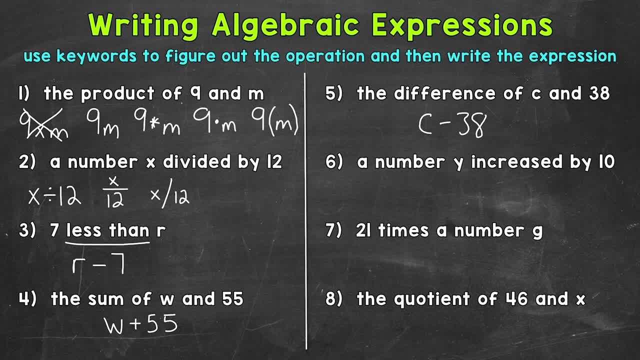 As opposed to number 3, where we switched that order. That's because we had that. less than So, pay attention to wording when it comes to these algebraic expressions. Number 6, we have a number y increased by 10.. Increased is our key word.